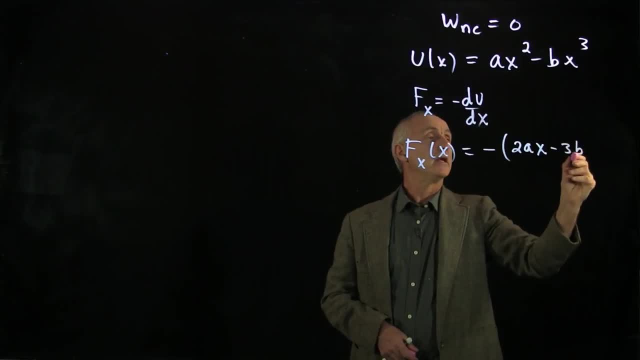 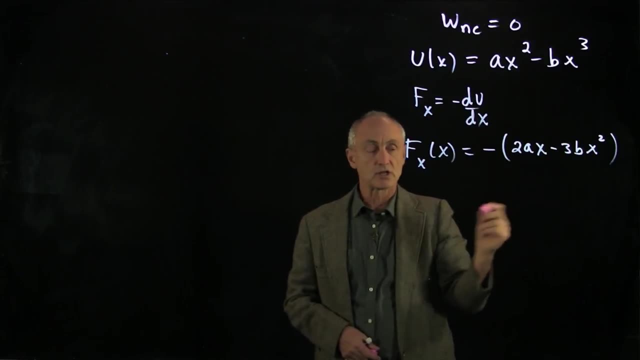 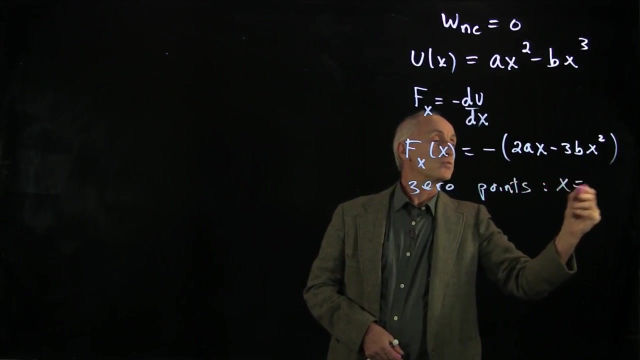 as the force goes: 2ax minus 3bx squared. Now we ask ourselves: where does this force vanish? So if we look at the zero points for the force, we can see immediately that there's one x equals 0.. The other one, if we said 2ax equals 3bx squared, tells us that we have another. 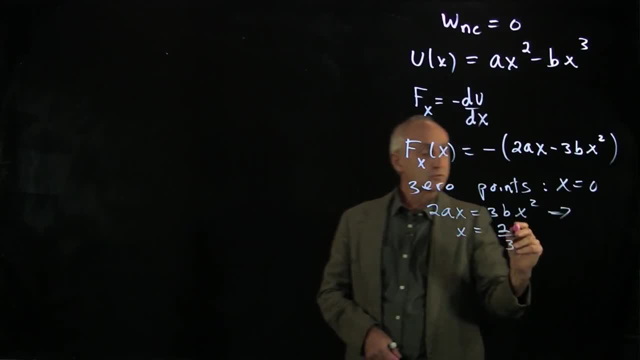 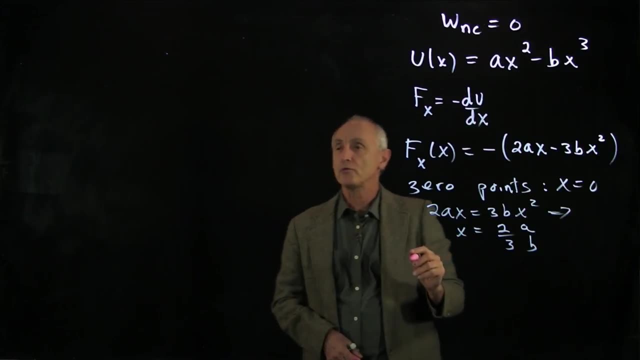 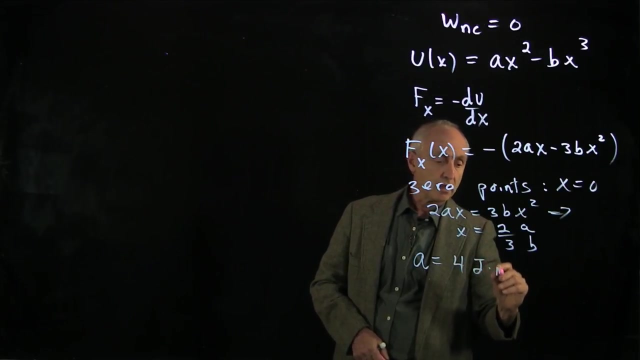 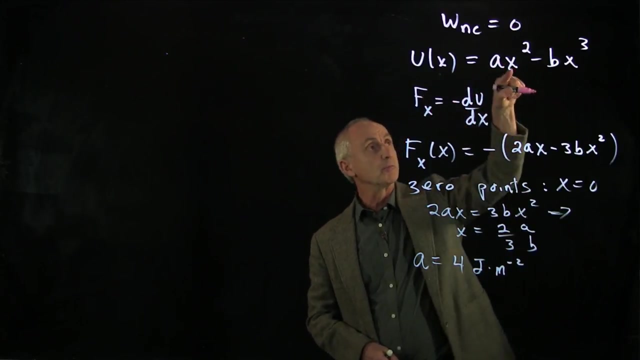 zero point at 2 thirds a over b. Now let's also, for our example, just put some numbers in first. So if we look at this simplicity, let's write this as 4 joules per meter squared for a. Why do we have meter squared? Well, the units of potential energy are joules, and we're 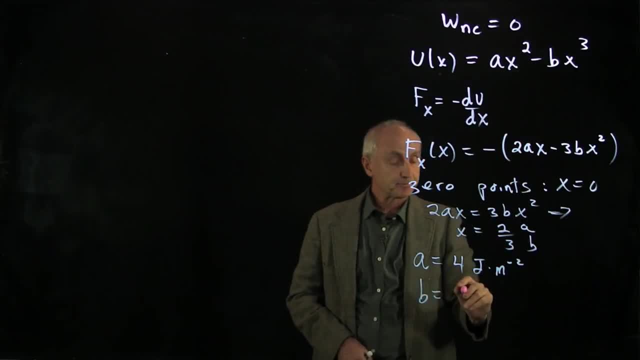 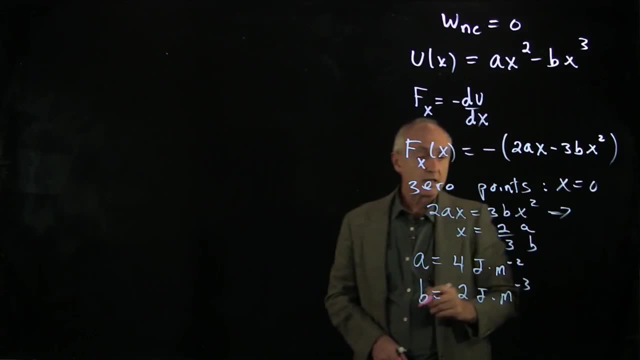 multiplying by x squared, And so you can see that b also we're going to write as 2 joules meter to the minus 3.. And if we put those numbers in we can see that we'll get 8 over 6.. 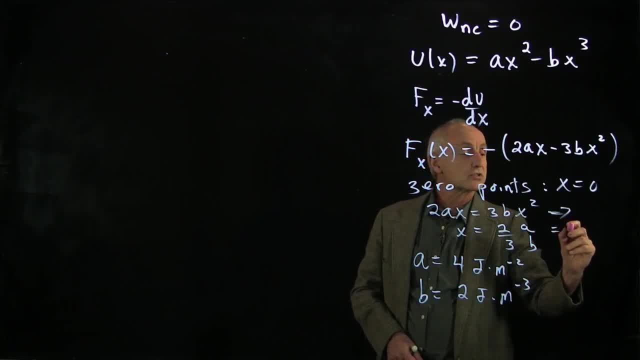 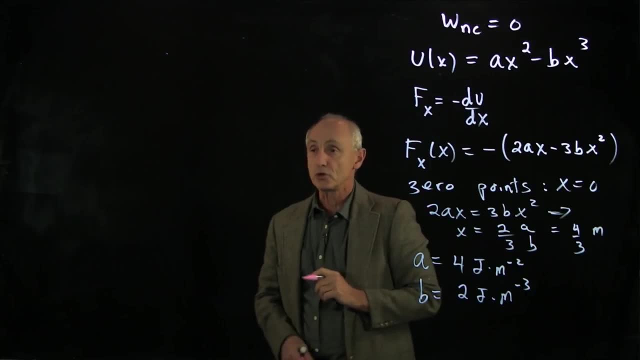 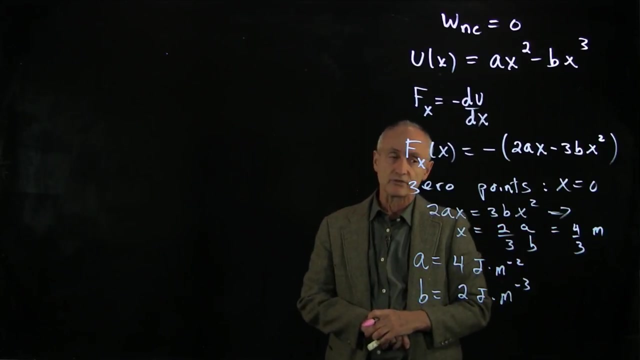 And 8 over 6. And 8 over 6.. And 8 over 6 is just 4 thirds, And that will be in meters where the other zero point is. So that's nice, but we'd like to know some properties of these zero points. 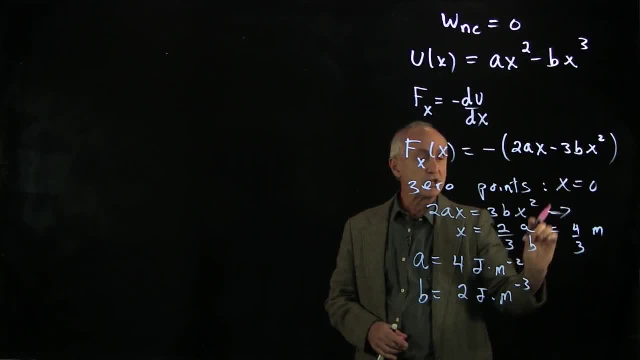 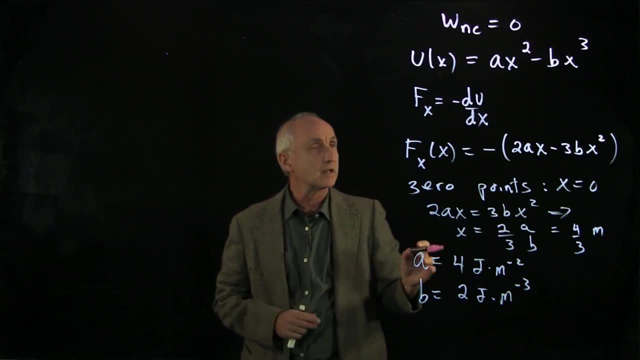 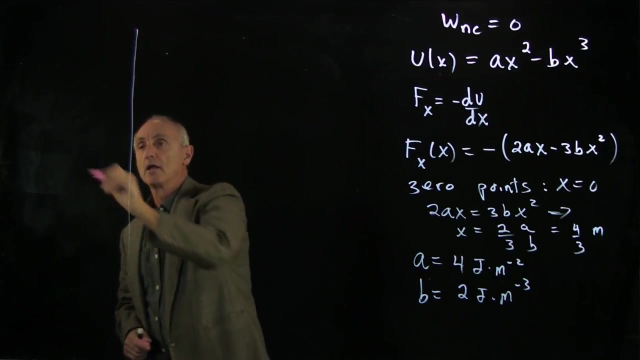 If we had a particle that we started with some energy at one zero point, where would it go? What would it do at the other point? So, in order to understand a little bit more detail about these zero points, let's make a plot of our potential energy: u of x versus x. 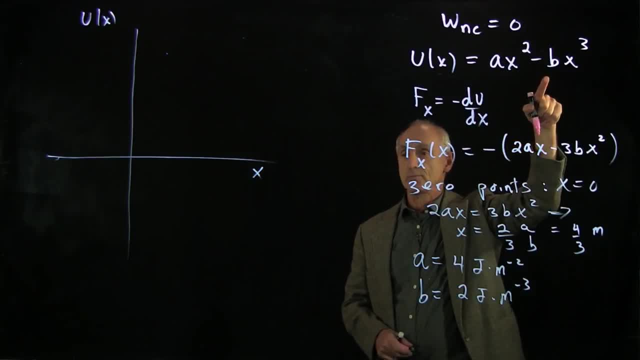 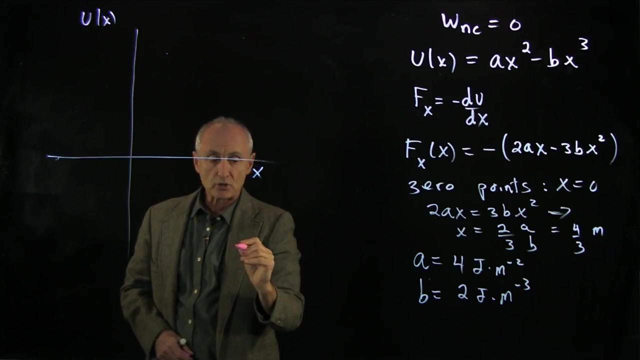 Now, to begin with, we want to ask ourselves how does this function behave? And for big values of x, the x cubed piece will dominate. And if we're positive x, we dominate with a negative value for potential energy, So our potential energy function goes off. 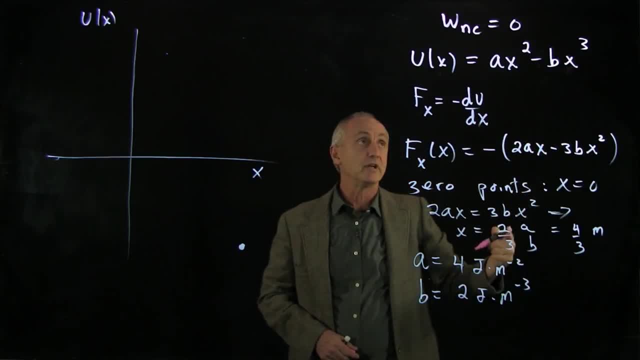 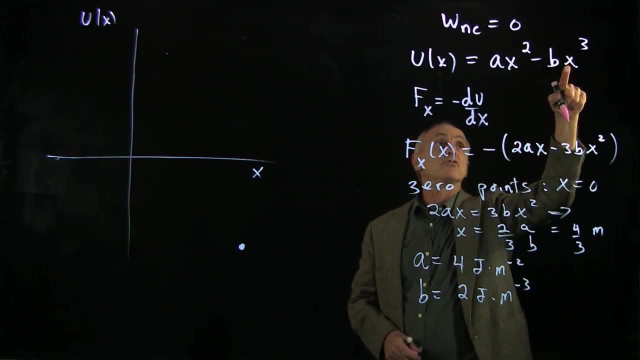 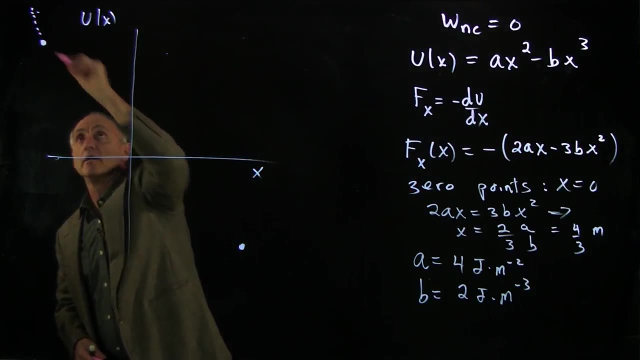 It goes off into negative infinity as x goes to infinity. Now, on the other side of the scale, the x cubed term will dominate for negative values of x. But this term is negative and that's negative. So up here it will go off to infinity in the positive direction. 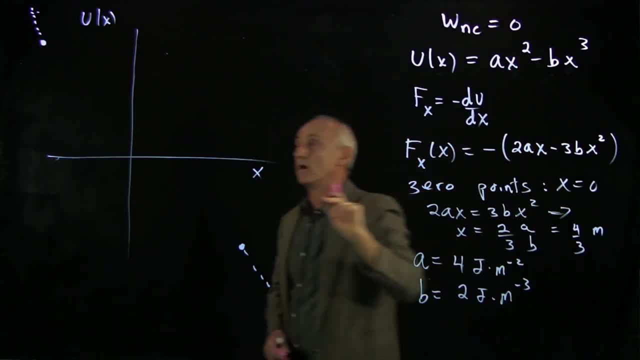 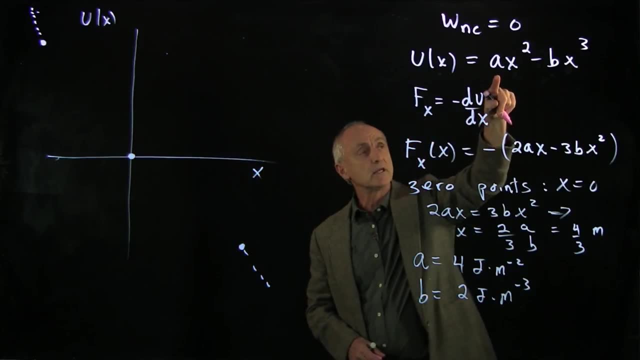 Now, where are the zeros of the potential function? There's one, obviously, one at x equals 0. So the values- it's not 100% obvious immediately, but 4x squared minus 2b, x cubed, If you set x equal to 2, 4 times 2 is 8.. 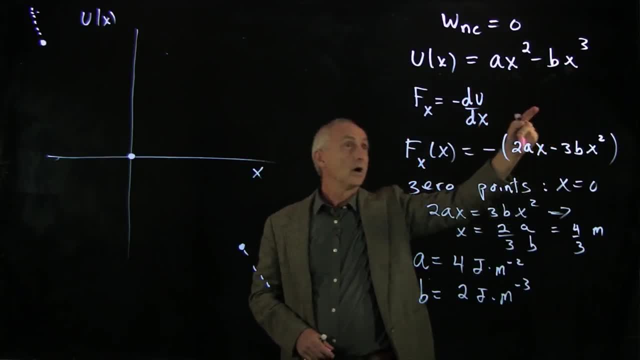 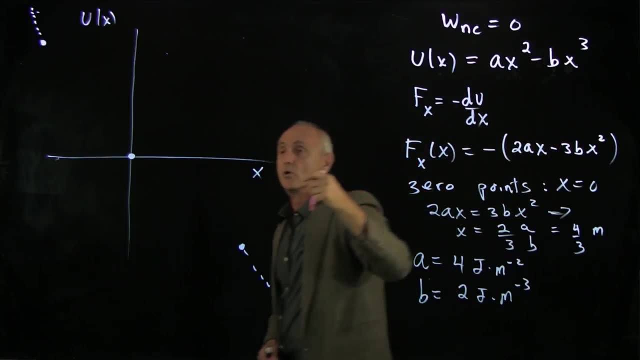 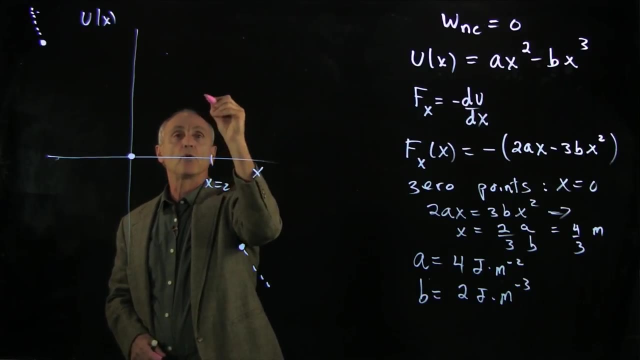 b 2 times 2, 4 times 4 is 16.. If b is 2 and x is 2, that's 16.. So we get a cancellation at x equals 2.. And so we have A point up here. 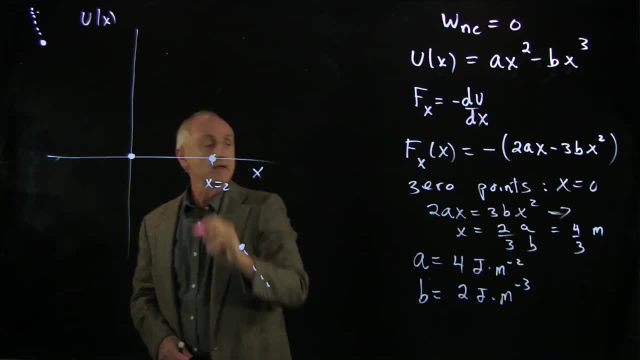 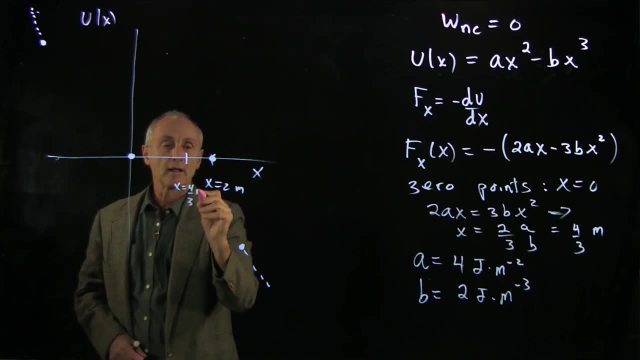 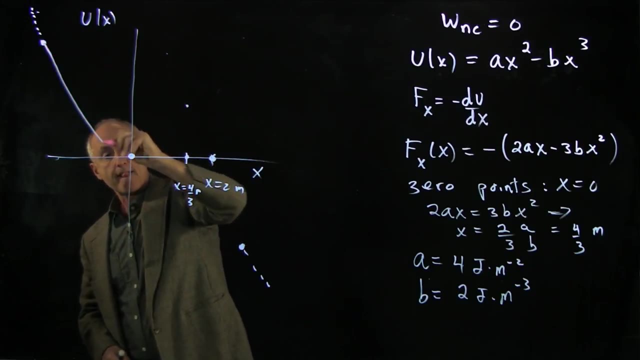 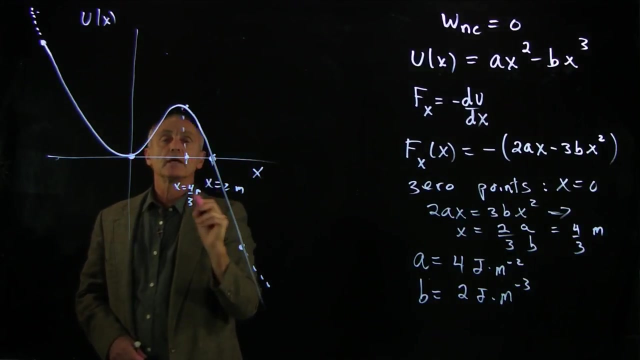 I'm sorry, that's our 0 point at x equals 2.. Now we said that the force at x equals 4 thirds had a 0. And so if we plot this function, it's going to look something like that. Now let's focus on these two points. 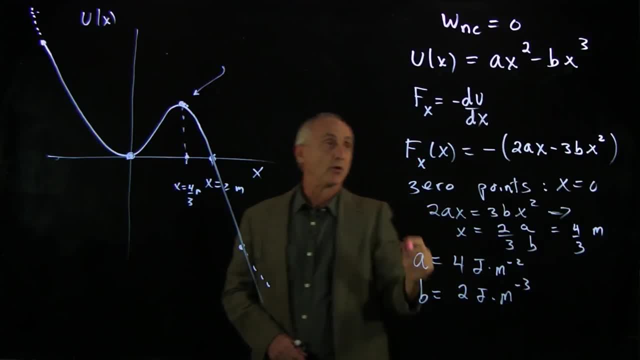 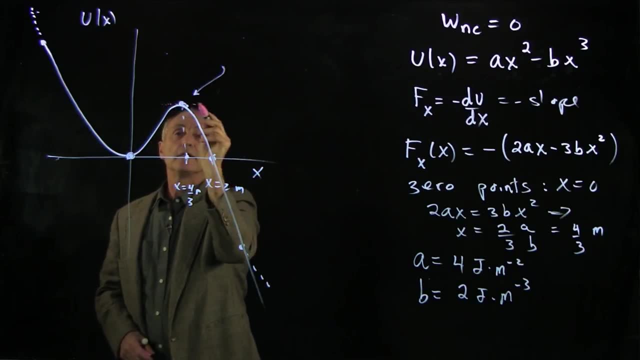 So we have these two points right here where our force is 0. Remember that this is minus the slope, And so we can see immediately that these two points have 0 slope, And so the force is 0 there. Notice, potential energy always depends on a reference point. 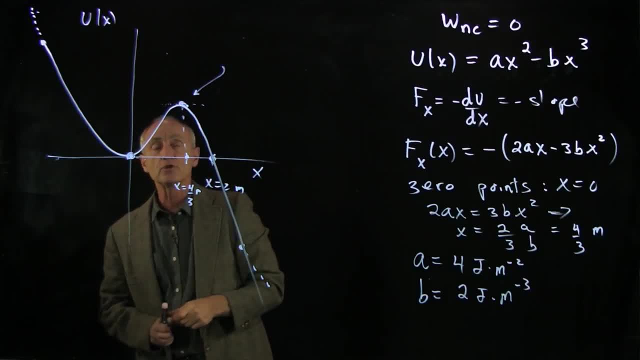 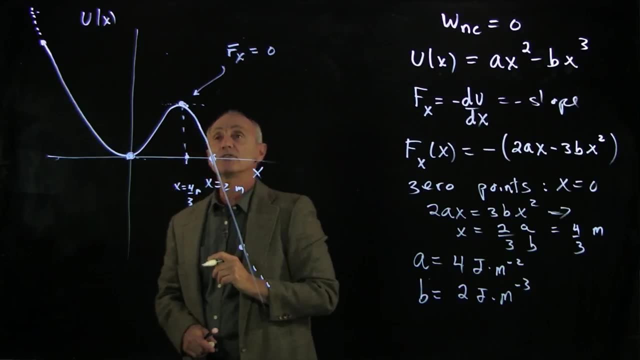 So whether the potential energy is 0 or not is not crucial, But the physical fact that the force is 0 there has physical meaning. So here this is one of our points. So we can see that the force at x is 0.. 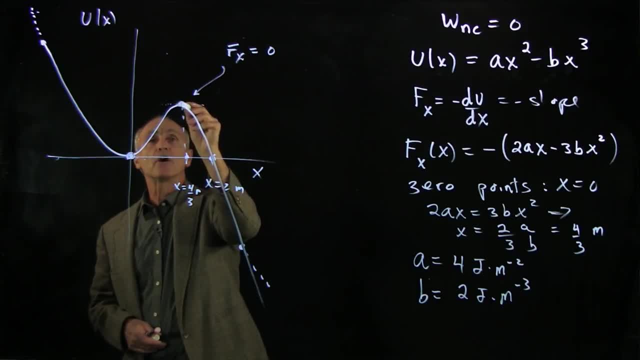 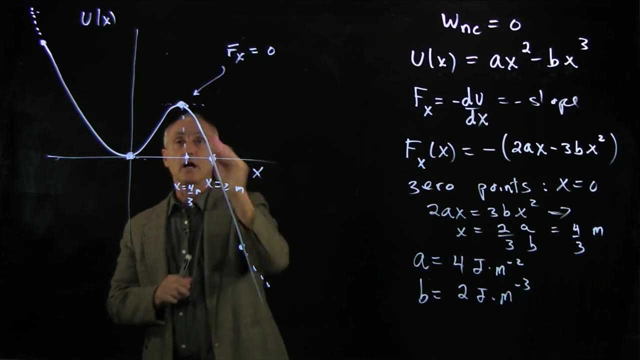 Now, what is the property of this point? Well, suppose we ask ourselves, if the particle were just displaced slightly from this position where the force is 0, which way would the force point? Well, in order to answer a question like that, we can look at the slopes on either side of this 0. 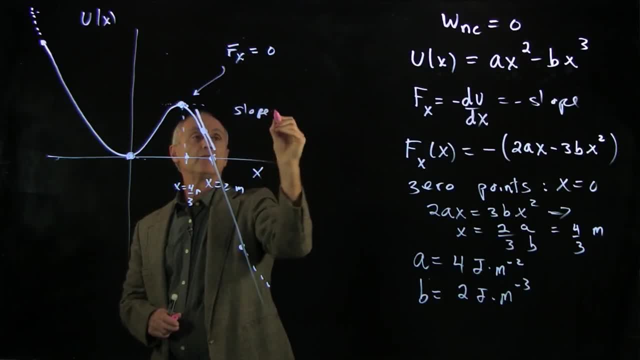 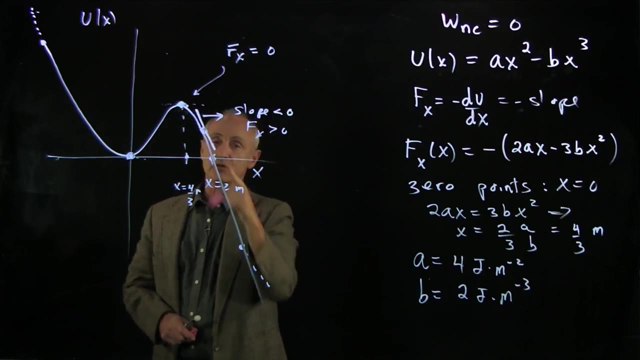 So over here the slope is negative But the force is minus the slope, So f of x is positive on this side, And so if a particle is displaced a little bit from this 0 point, it moves off to the right And it will continue to feel a force in this direction.